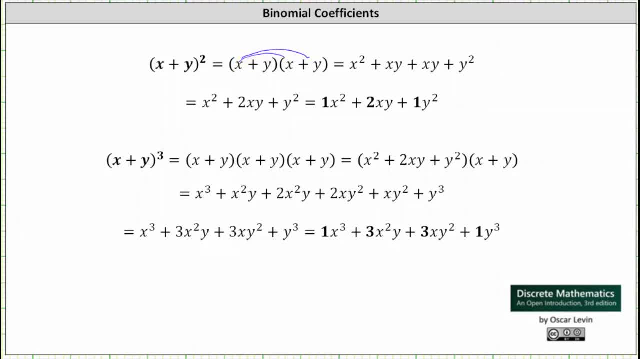 where we distribute the x from the first binomial and then we distribute the y from the first binomial. This gives us x squared plus xy plus xy plus y squared, which simplifies to x squared plus 2xy plus y squared, which I've written here to emphasize all the coefficients, And now it's cube: x plus y. 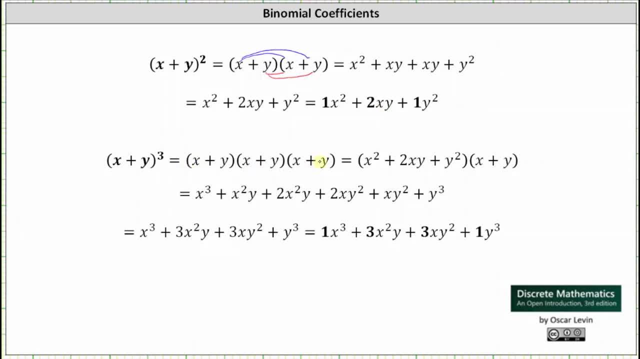 There are no shortcuts. We have three factors of x plus y, but we do know x plus y times. x plus y is x squared plus 2xy plus y, squared from squaring x plus y. and now we have to multiply by x plus y. 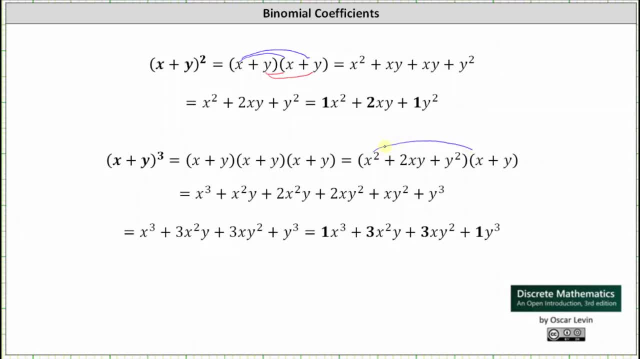 Which means we distribute the x squared, we distribute the 2xy and we distribute the y squared. This gives us x cubed plus x squared y, plus 2x squared y, plus 2xy squared plus xy squared plus y cubed, which simplifies to x cubed plus 3x squared y. 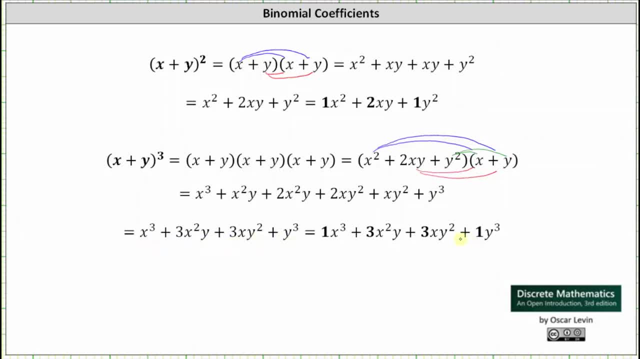 plus 3xy squared plus y cubed, which I've written here to emphasize all of the coefficients. But there's a much easier way to determine a binomial coefficient. For example, if you wanted to find the coefficient of x cubed, y squared in the expansion of the fifth. 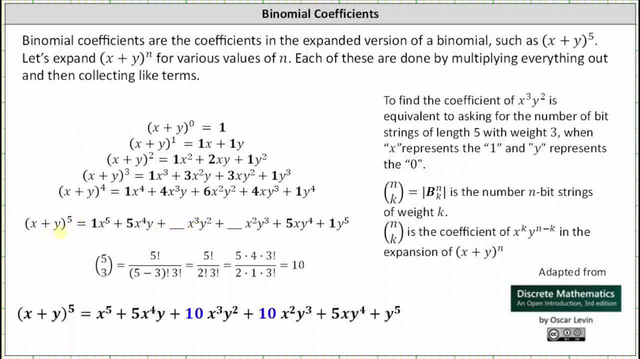 power of x plus y. this is equivalent to asking for the number of bit strings of length 5 with weight 3, where x represents the 1 and the y represents the 0. So because we have x cubed, we have three ones, and because we have y squared, we have two zeros, which again does give a bit. 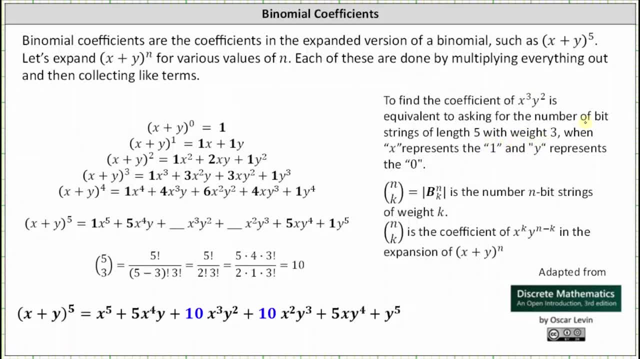 string of length 5 with weight 3.. And we can determine the number of bit strings of length 5 with weight 3 by evaluating a combination. Remember, the number of n-bit strings of weight k is equal to n choose k and therefore n choose k is also the coefficient of x to the power of k. 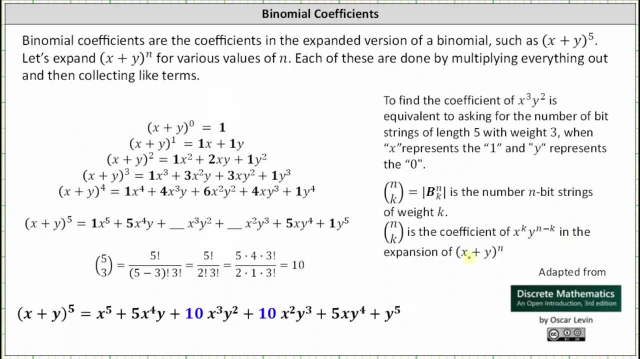 y to the power of n minus k in the expansion of the nth power of x plus y. As an example, if we're looking at the expansion of the fifth power of x plus y, notice n is equal to 5 and because we're looking for the coefficient of x to the third, y squared. 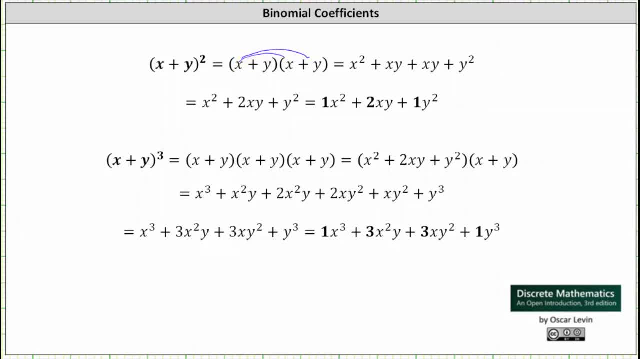 where we distribute the x from the first binomial and then we distribute the y from the first binomial. This gives us x squared plus xy plus xy plus y squared, which simplifies to x squared plus 2xy plus y squared, which I've written here to emphasize all the coefficients, And now it's cube: x plus y. 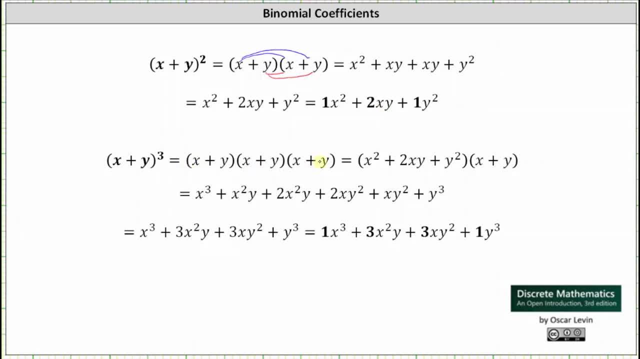 There are no shortcuts. We have three factors of x plus y, but we do know x plus y times. x plus y is x squared plus 2xy plus y, squared from squaring x plus y. and now we have to multiply by x plus y. 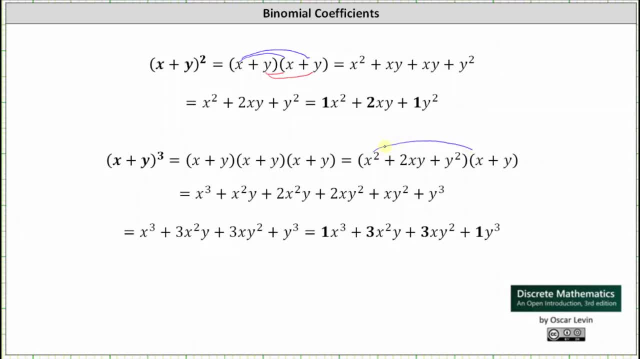 Which means we distribute the x squared, we distribute the 2xy and we distribute the y squared. This gives us x cubed plus x squared y, plus 2x squared y, plus 2xy squared plus xy squared plus y cubed, which simplifies to x cubed plus 3x squared y. 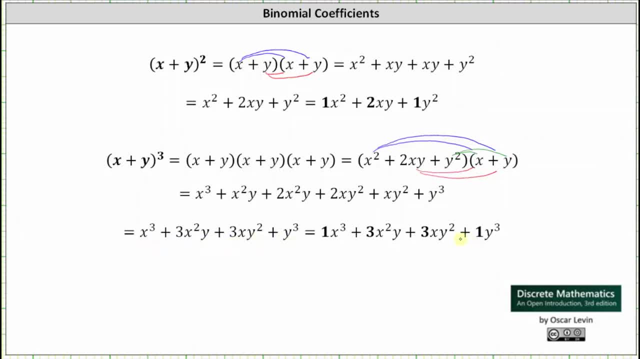 plus 3xy squared plus y cubed, which I've written here to emphasize all of the coefficients. But there's a much easier way to determine a binomial coefficient. For example, if you wanted to find the coefficient of x cubed, y squared in the expansion of the fifth. 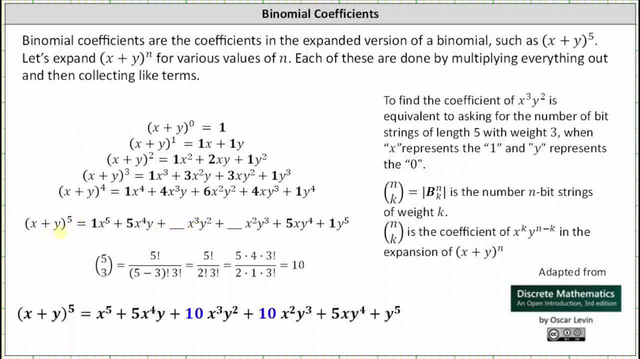 power of x plus y. this is equivalent to asking for the number of bit strings of length 5 with weight 3, where x represents the 1 and the y represents the 0. So because we have x cubed, we have three ones, and because we have y squared, we have two zeros, which again does give a bit. 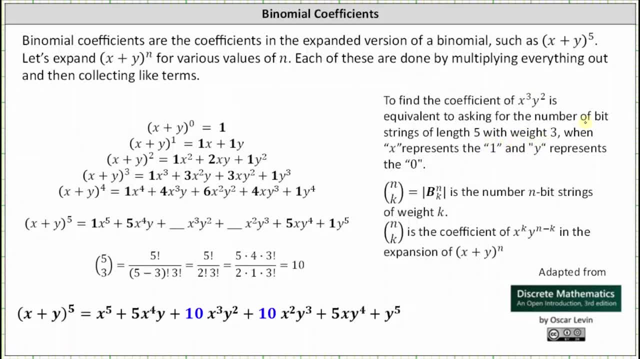 string of length 5 with weight 3.. And we can determine the number of bit strings of length 5 with weight 3 by evaluating a combination. Remember, the number of n-bit strings of weight k is equal to n choose k and therefore n choose k is also the coefficient of x to the power of k. 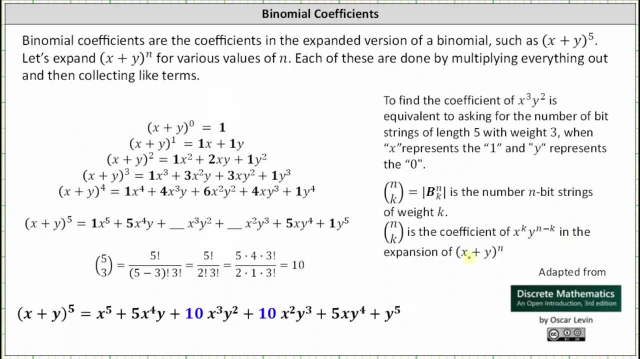 y to the power of n minus k in the expansion of the nth power of x plus y. As an example, if we're looking at the expansion of the fifth power of x plus y, notice n is equal to 5 and because we're looking for the coefficient of x to the third, y squared. 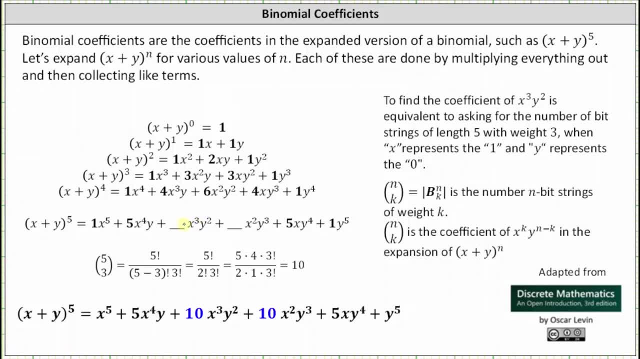 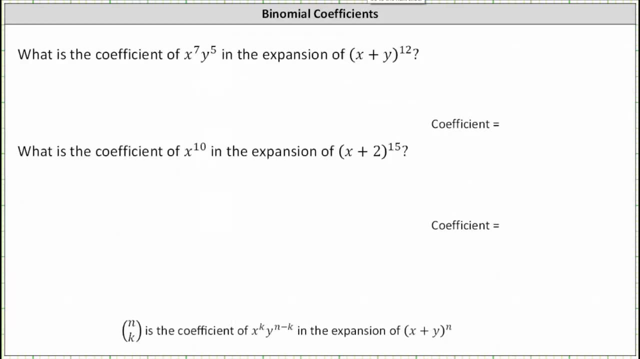 k is equal to 3. this indicates the coefficient is 5 choose 3, which is equal to 10.. And the coefficient of x squared y cubed is also 10, because 5 choose 2 is also 10.. Let's take a look at two more examples. Let's determine the coefficient of x to the seventh. 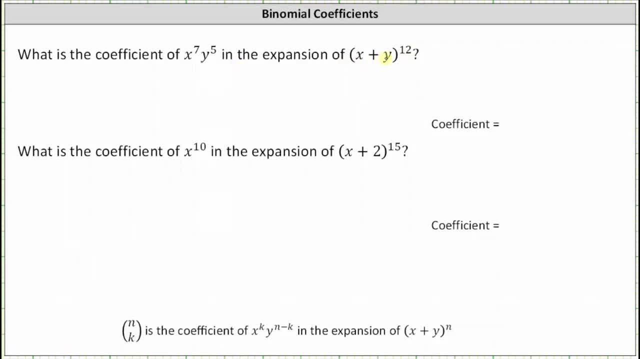 y to the fifth in the expansion of the 12th power of x plus y. So first notice that n, exponent on the quantity x plus y is 12 and k the exponent on x is 7.. So let's first find the x to the seventh, y to the fifth term, and then we'll give the coefficient. So we have x to the. 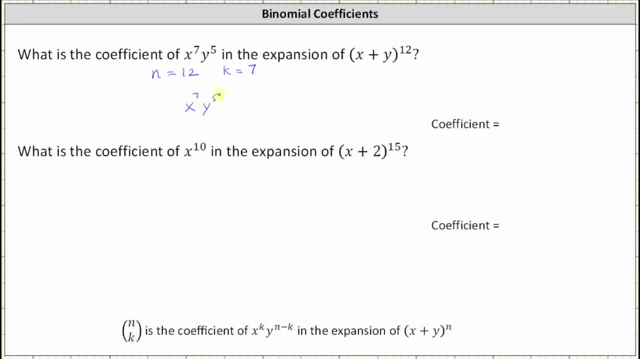 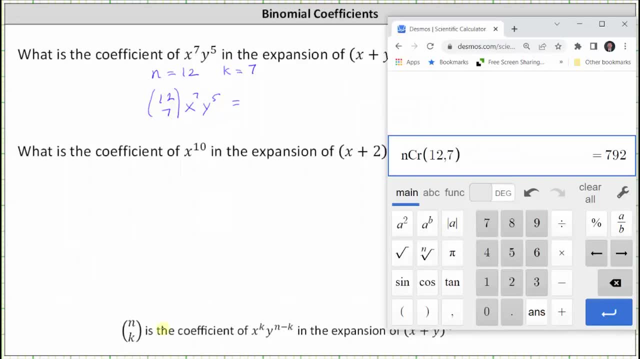 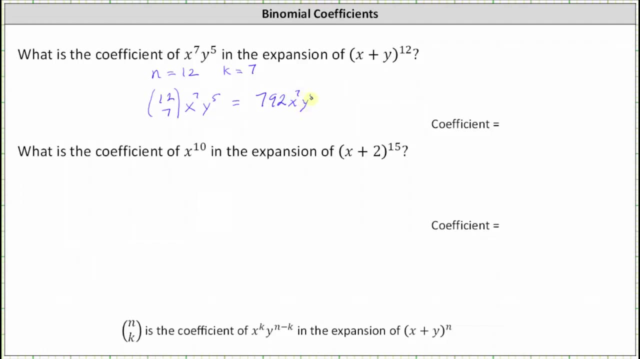 seventh, y to the fifth, and therefore the coefficient is n. choose k, which is 12, choose 7.. 12 to 7 is equal to 792, and therefore the term is 792.. x to the seventh, y to the fifth, the coefficient is 792.. 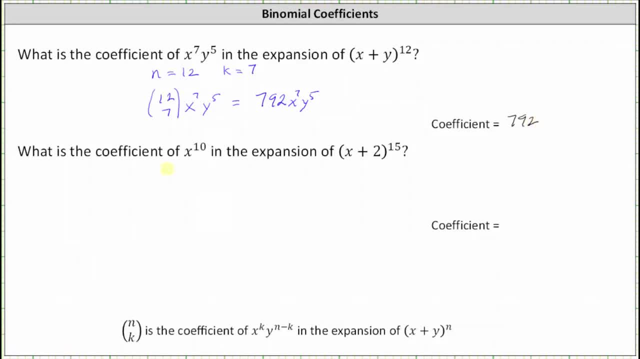 And let's look at the second example, which is a little bit different. What is the coefficient of x to the 10th in the expansion of the 15th power of x plus 2?? So notice, here we have x plus 2 and 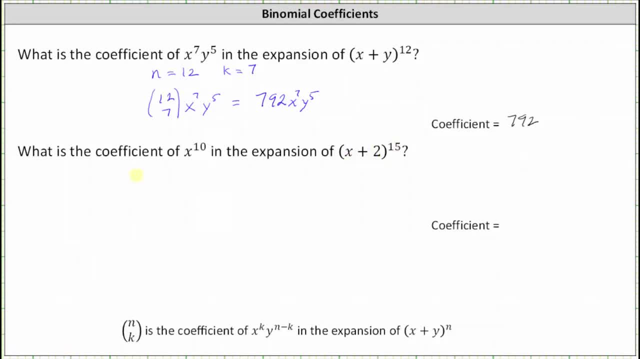 not x plus y. So, to begin, n is equal to 15 and because we're looking for the coefficient of x to the 10th, k is equal to 10.. So let's find the x to the 10th power of x plus 2.. So let's find the. 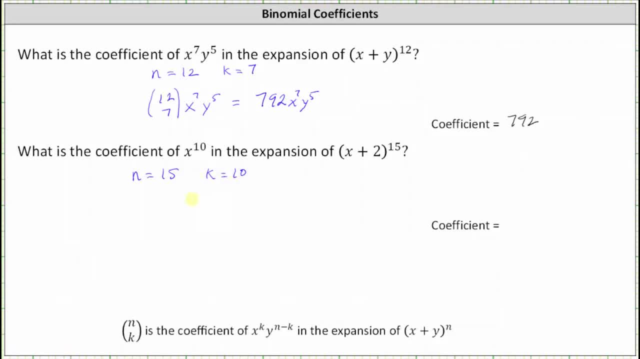 x to the 10th term and then we'll give the coefficient. So again, we're going to have x to the 10th. but looking at our formula, notice how we also have y, the power of n minus k, and our y value is now positive 2.. So we do have to raise 2 to the power of n minus k, and minus k is 15. 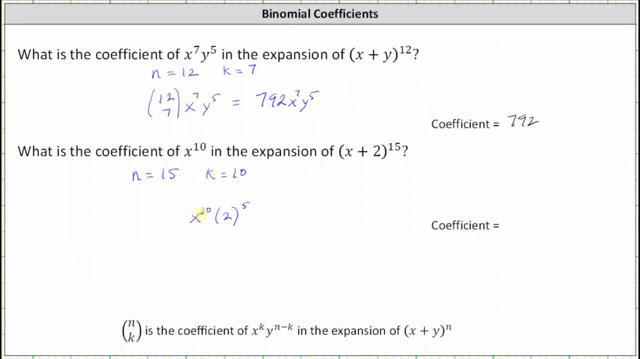 minus 10, which is 5.. The sum of these exponents should always equal n, and then the combination is going to be again n choose k, which is 15 choose 10.. So notice, in this case 15 choose 10 is not going to be the coefficient, because we also need to multiply by 2 to the 5th. 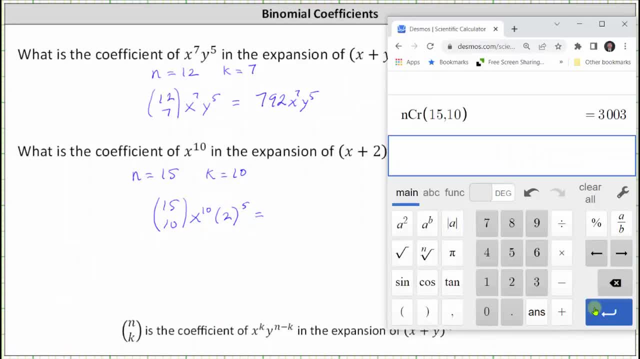 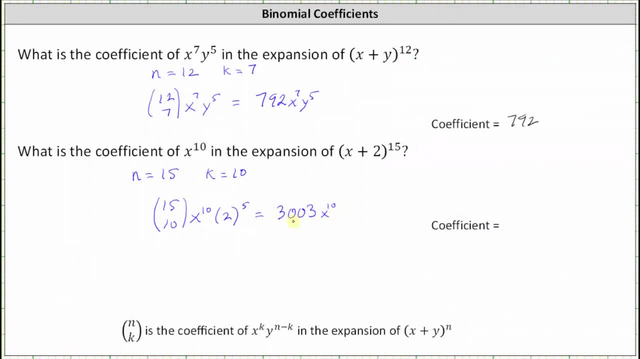 So let's first determine: 15 choose 10.. 15 choose 10 is 3003.. This gives us 3003 times x to the 10th, times 2 to the 5th, which is 32, which means the coefficient is going to be 3003 times 32. 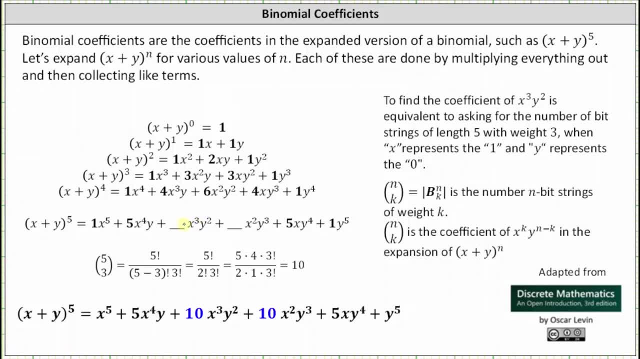 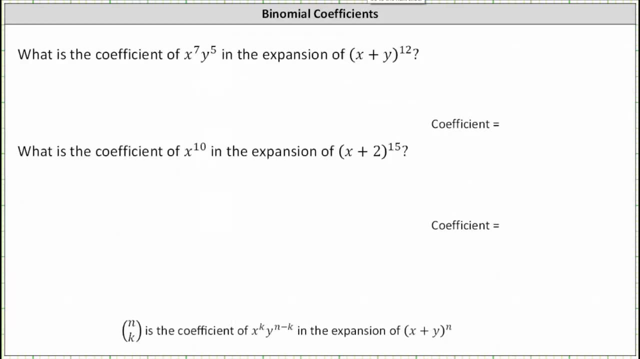 k is equal to 3. this indicates the coefficient is 5 choose 3, which is equal to 10.. And the coefficient of x squared y cubed is also 10, because 5 choose 2 is also 10.. Let's take a look at two more examples. Let's determine the coefficient of x to the seventh. 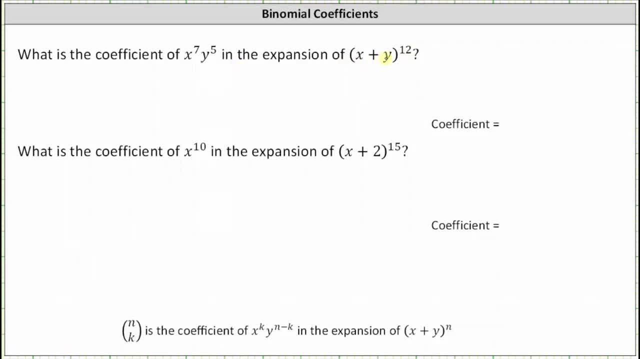 y to the fifth in the expansion of the 12th power of x plus y. So first notice that n, exponent on the quantity x plus y is 12 and k the exponent on x is 7.. So let's first find the x to the seventh, y to the fifth term, and then we'll give the coefficient. So we have x to the. 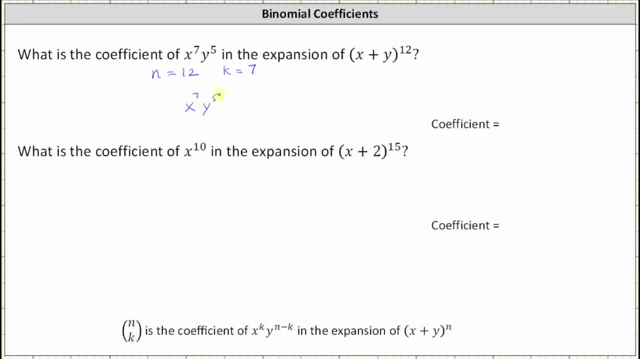 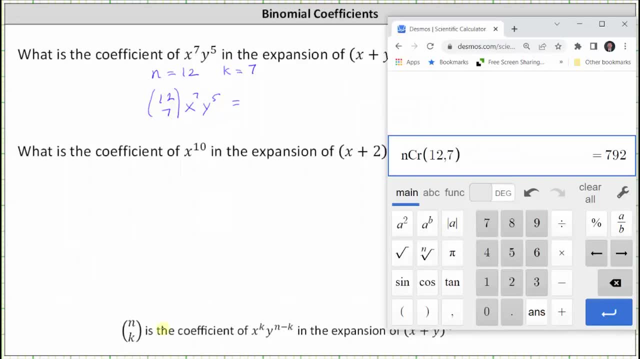 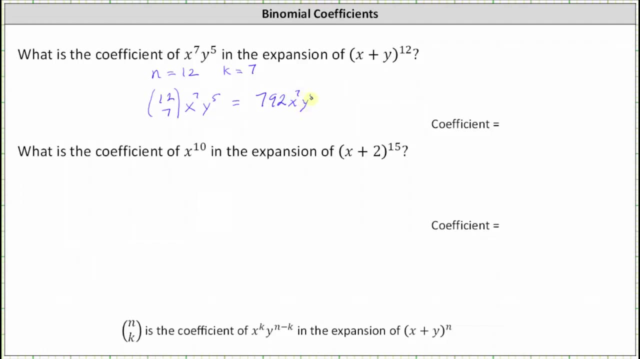 seventh, y to the fifth, and therefore the coefficient is n. choose k, which is 12, choose 7.. 12 to 7 is equal to 792, and therefore the term is 792.. x to the seventh, y to the fifth, the coefficient is 792.. 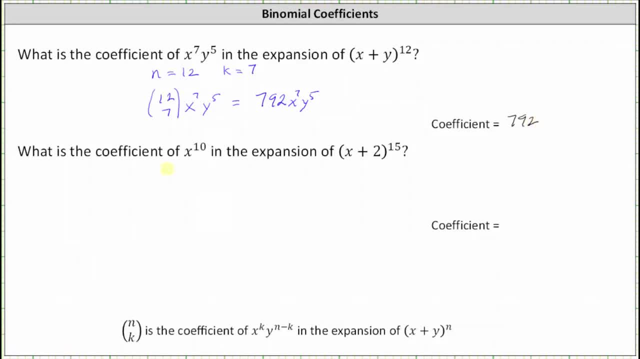 And let's look at the second example, which is a little bit different. What is the coefficient of x to the 10th in the expansion of the 15th power of x plus 2?? So notice, here we have x plus 2 and 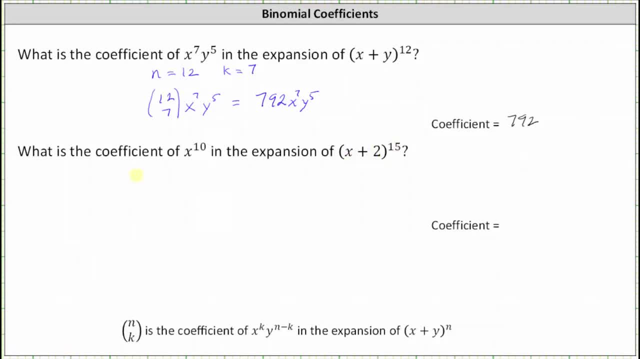 not x plus y. So, to begin, n is equal to 15 and because we're looking for the coefficient of x to the 10th, k is equal to 10.. So let's find the x to the 10th power of x plus 2.. So let's find the. 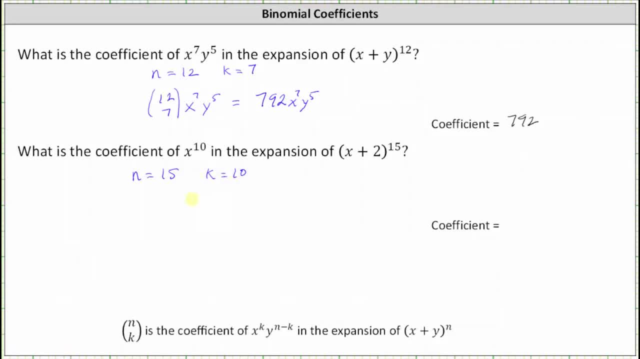 x to the 10th term and then we'll give the coefficient. So again, we're going to have x to the 10th. but looking at our formula, notice how we also have y, the power of n minus k, and our y value is now positive 2.. So we do have to raise 2 to the power of n minus k, and minus k is 15. 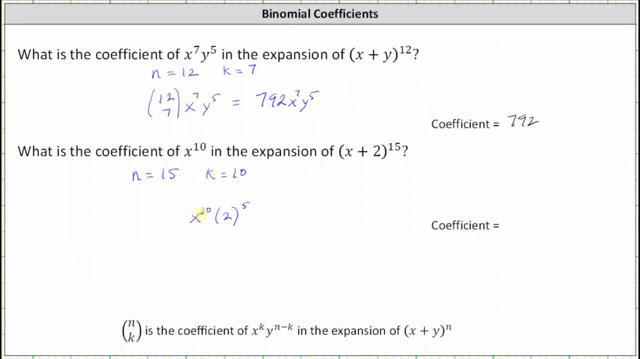 minus 10, which is 5.. The sum of these exponents should always equal n, and then the combination is going to be again n choose k, which is 15 choose 10.. So notice, in this case 15 choose 10 is not going to be the coefficient, because we also need to multiply by 2 to the 5th. 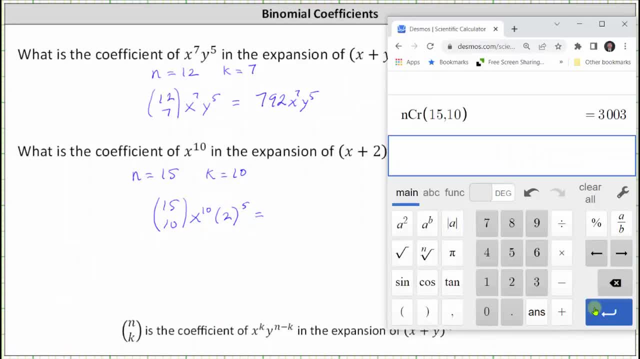 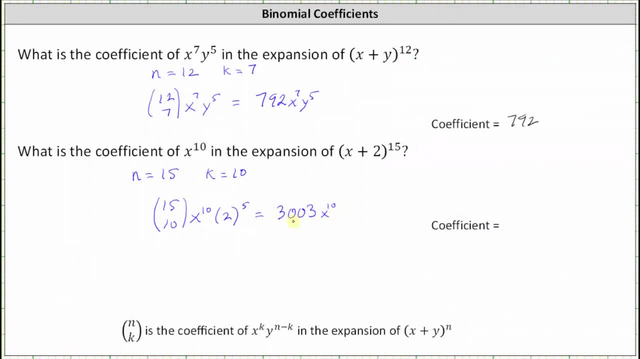 So let's first determine: 15 choose 10.. 15 choose 10 is 3003.. This gives us 3003 times x to the 10th, times 2 to the 5th, which is 32, which means the coefficient is going to be 3003 times 32.